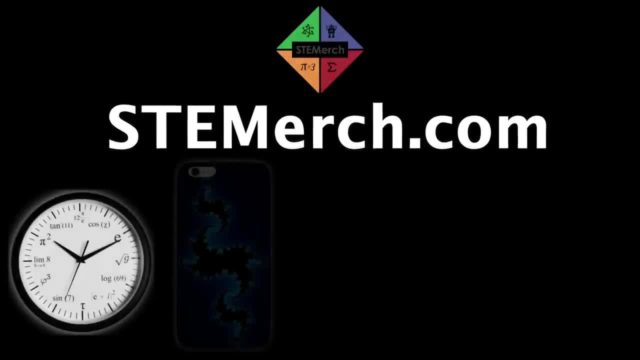 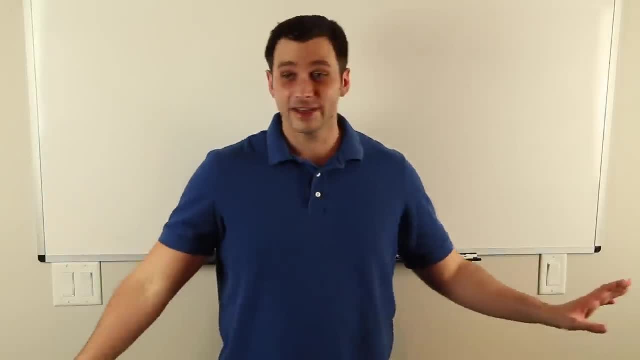 This video is brought to you by the newly launched stem merch store. more on that and some of the products we have. after the skit. We got this here. everyone else have a test, we all good, Okay, you guys have exactly one hour to finish. you can begin. 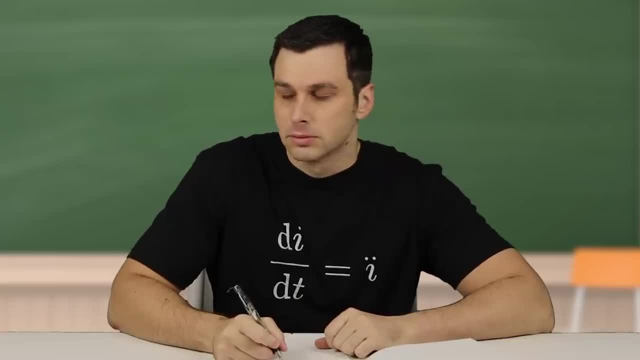 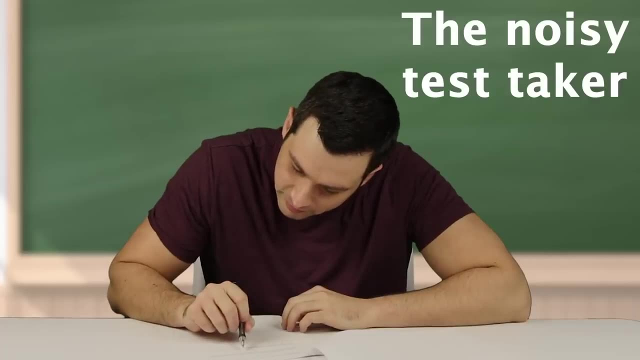 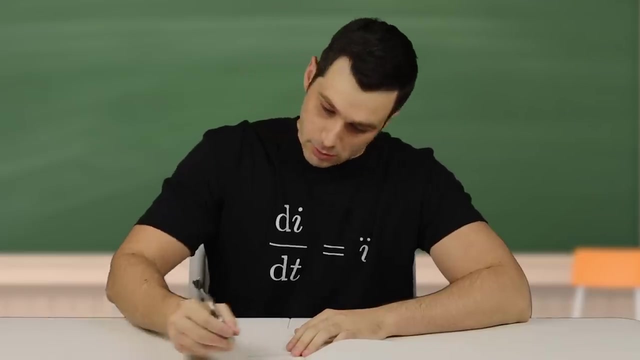 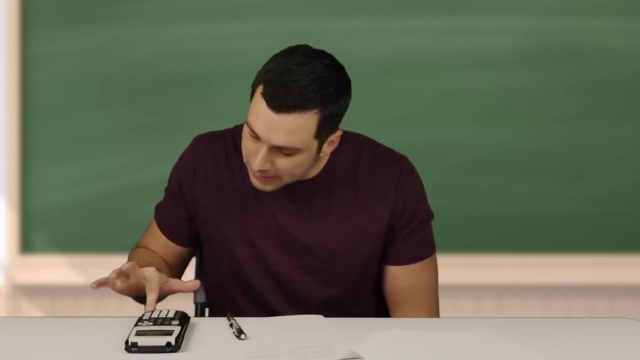 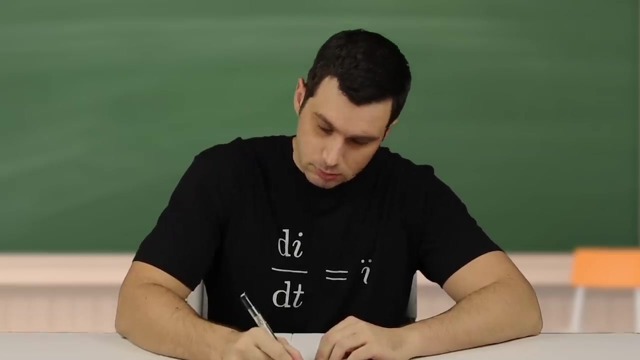 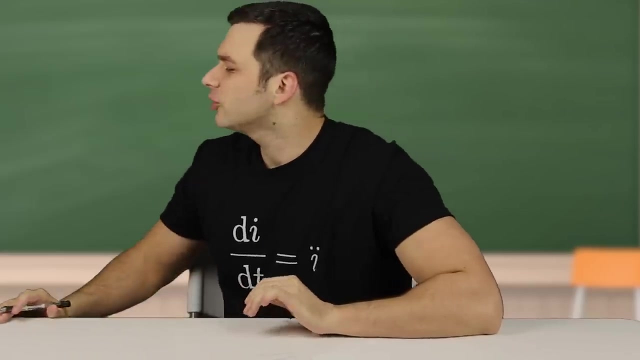 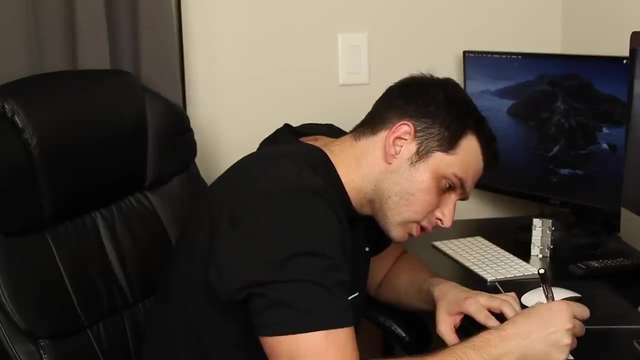 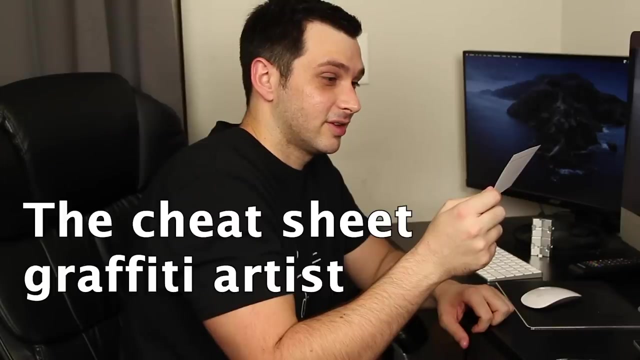 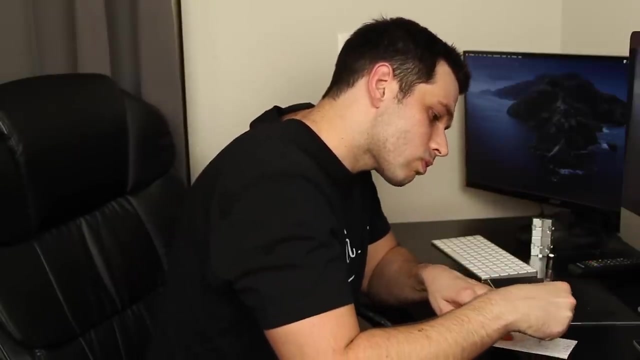 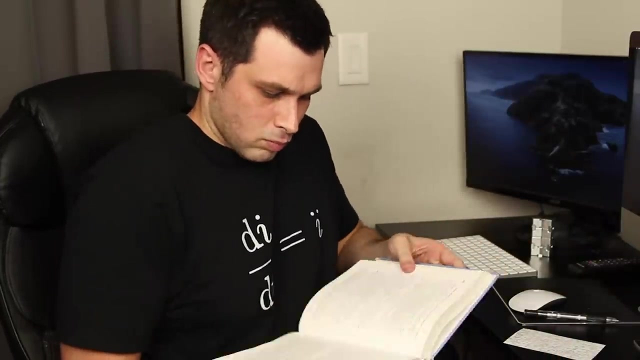 now. Oh, Shut the up. thank you You. This is a blank canvas. Oh, I can easily fit this equation here. You know, if I kind of wind the equation through the gaps, it totally fits. Okay, not even in this class. but better put some of these equations on here, just in case. 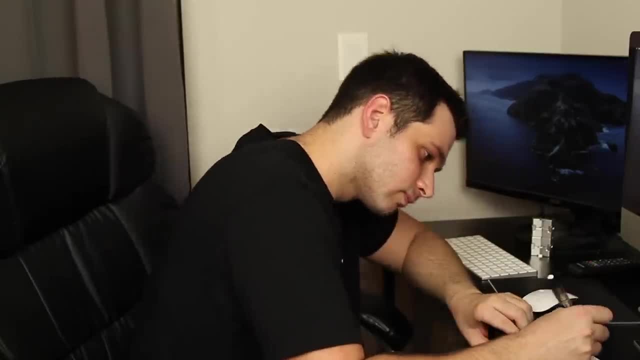 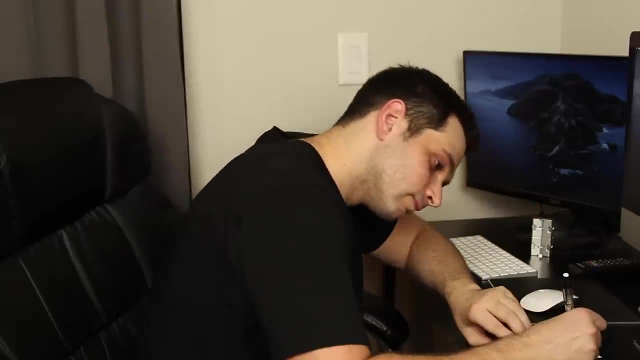 Never seen that before. better put it on the note card. Hmm, should I put F equals ma on here? I mean, I know it by heart, But I might forget it for some reason during the test. better put it on the note card. This is gonna be so easy to read on test day. 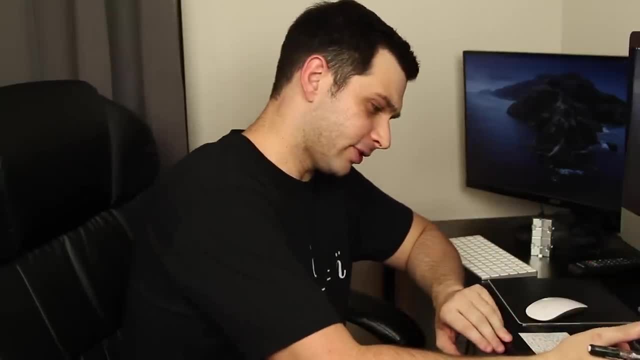 Should I put Schrodinger's equation on the cheat sheet for our dynamics- final No, you don't need to know Schrodinger's equation for that. I'm gonna put Schrodinger's equation on the cheat sheet for our dynamics- final Oh. 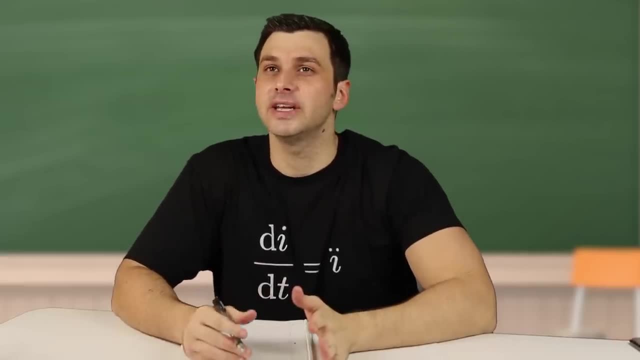 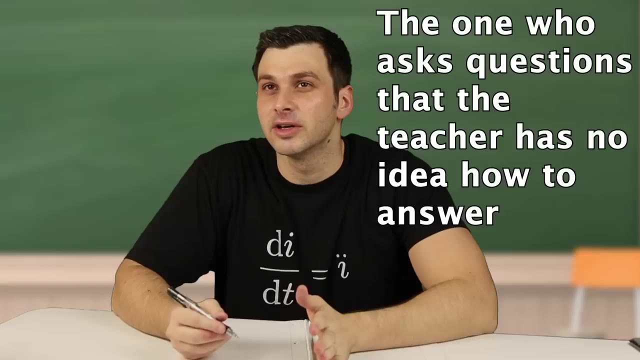 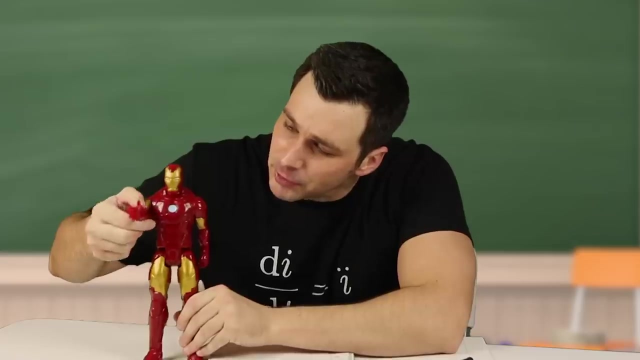 Yeah, um, so with that circuit, Would it have been used in Ironman's suit, an Iron man suit Like in that one scene where he was all like pew, pew, pew? Then the goop lady was all like: oh no, help me. and he was all like pew, pew, pew. 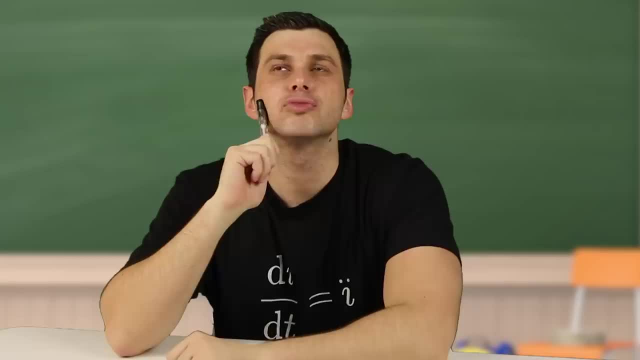 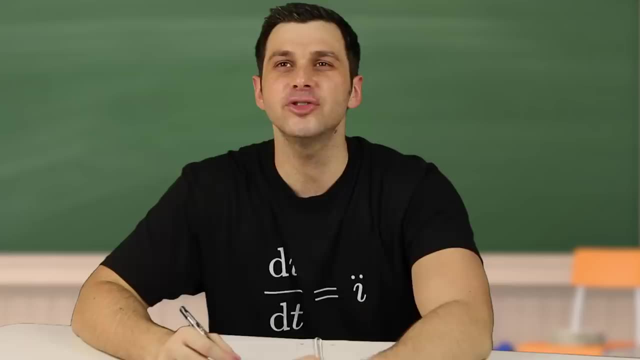 Yeah, would that circuit have been used there? So would the net force on the centre beam still be zero if the bridge were at the center of a black hole? How do you solve Navier-Stokes? I could use a million bucks, so could planes still-. 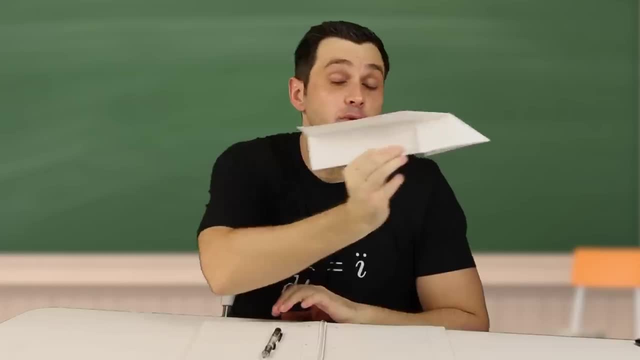 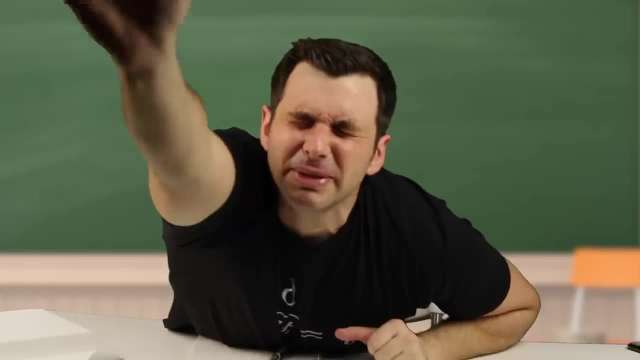 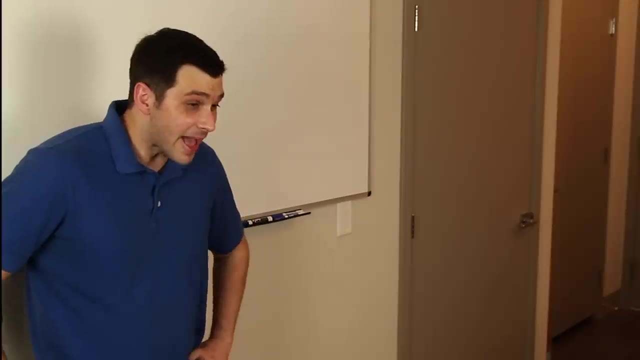 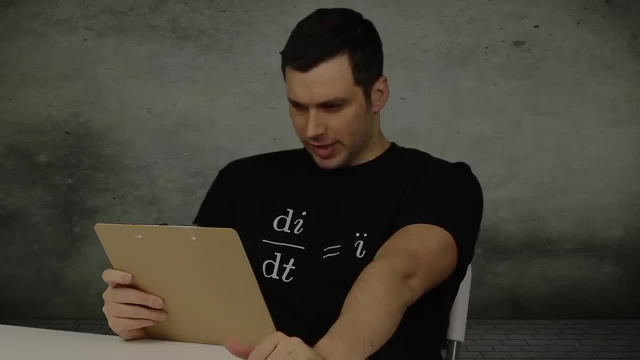 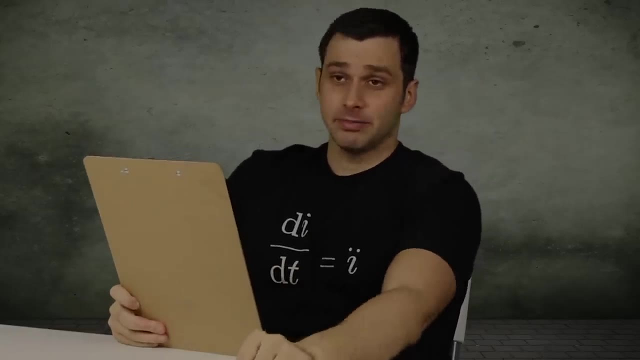 Well, I'll see you guys on Monday. So how'd you do it? I don't know. I guess I just got lucky. Okay, let's look at the facts. Let's look at the facts. After the midterm, I find you in the dorm. 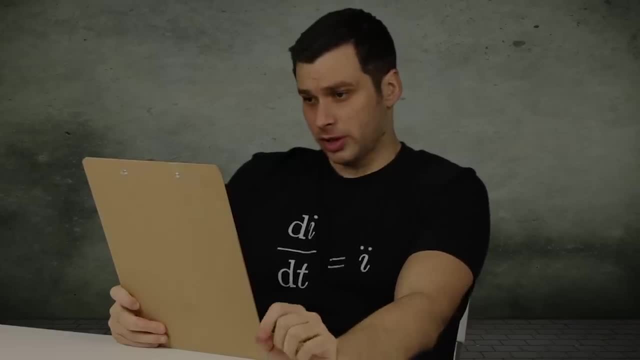 ask you how you think you did. You say, and I quote: dude did so bad, would be lucky if I got even one question right. Honestly, didn't even study for that test. Then you pull the highest grade in the class. 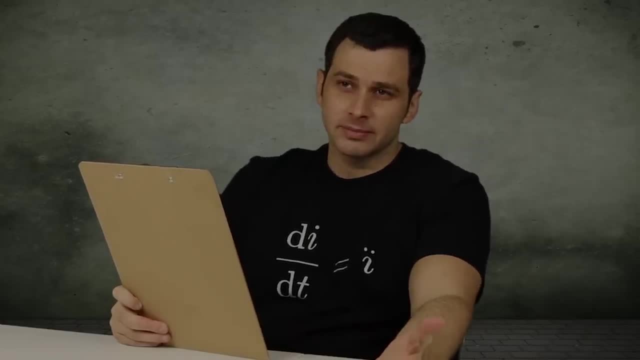 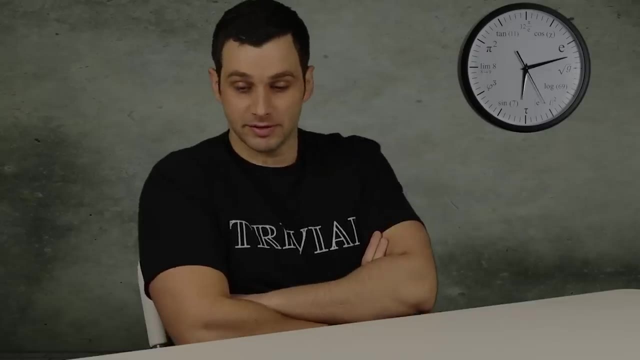 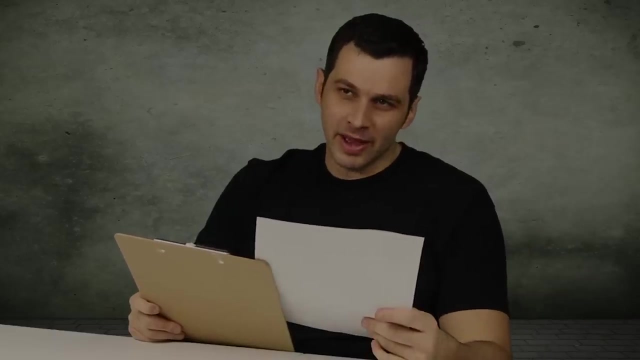 Now how do you explain that? Maybe this stuff just just comes naturally to me or something? Oh yeah, yeah, yeah, yeah yeah. Root locus blocks- they just come naturally to you, right? Do you think anyone's gonna buy that? 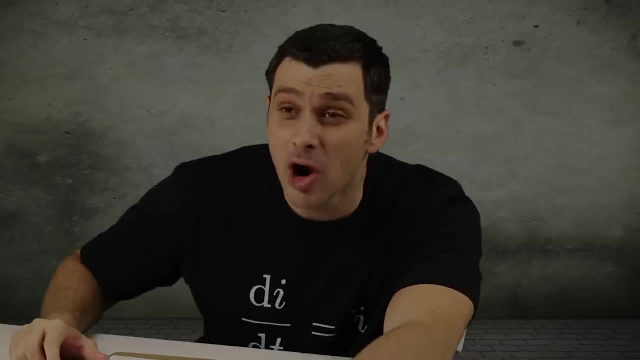 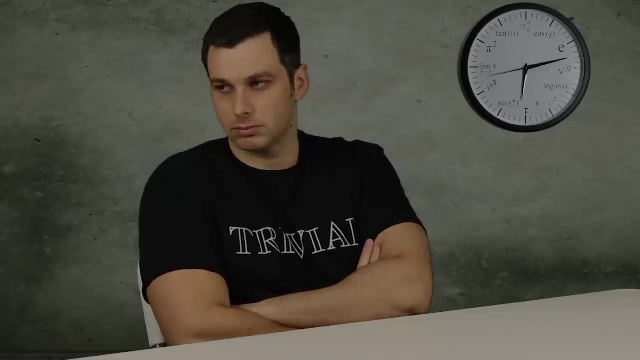 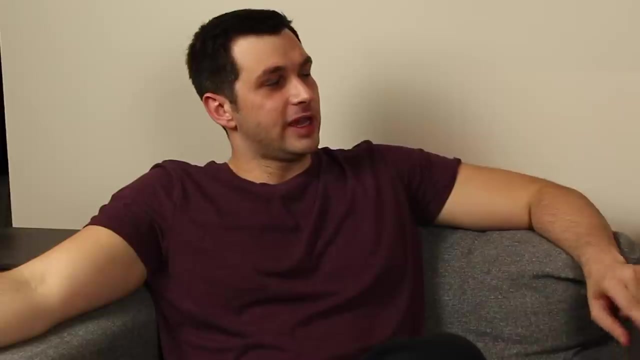 I think a jury of my peers will understand. Your peers hate you, bro. I got 12 angry men ready to beat the out of you because they actually studied for their test and barely passed with the curve that you ruined. Yeah. so I've been entering at NASA since I was three. 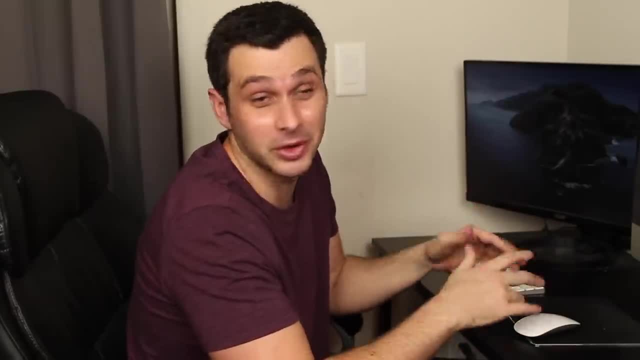 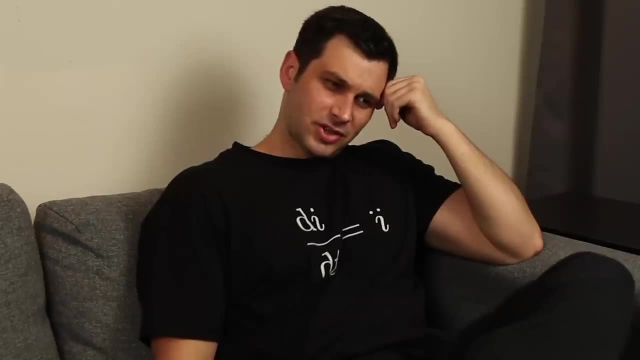 So yeah, well, you were coding hello world. I was an intern coding hello world of Warcraft, right? I mean, like that was me. What are you doing for your final lab project? I'm not sure I was thinking of maybe, dude, that's so cool. 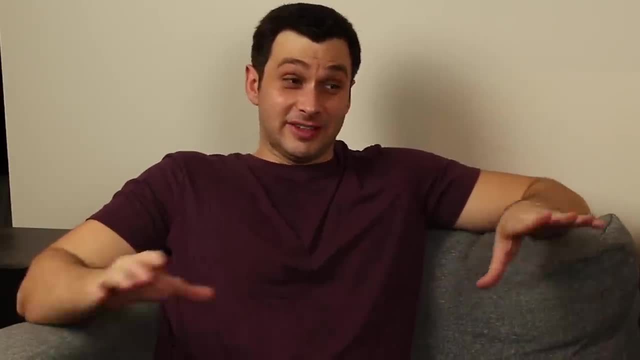 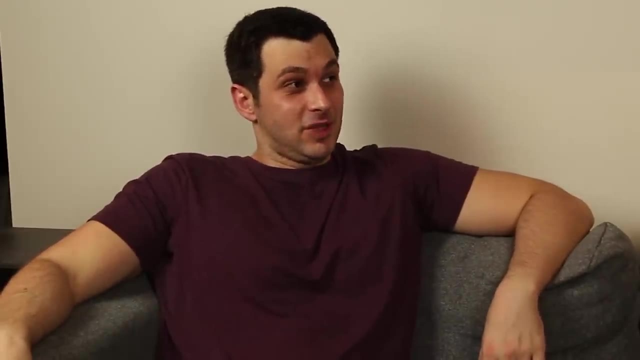 Oh, what am I working on? Well, I think I'm gonna make like a drone that has a sensor on it that can see through walls. There'll also be a lightsaber attached to it, So like: yeah, Sorry, what were you working on again? 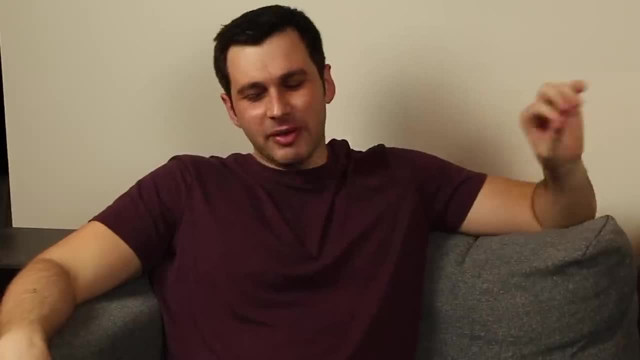 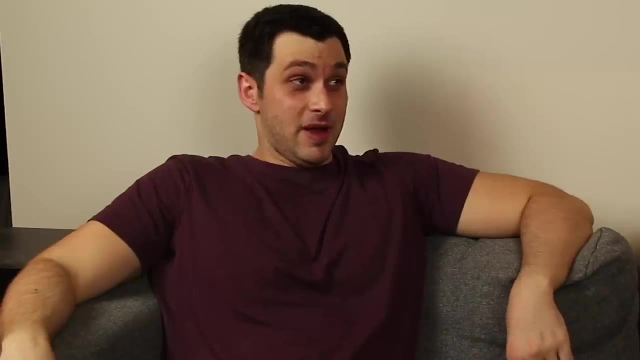 Right, yeah, I was gonna design something either on the computer, Not even listening. I'll be able to sell my drone to Boeing when I'm done with it and then I'll use that money to buy Boeing. But yeah, your project sounds cool. 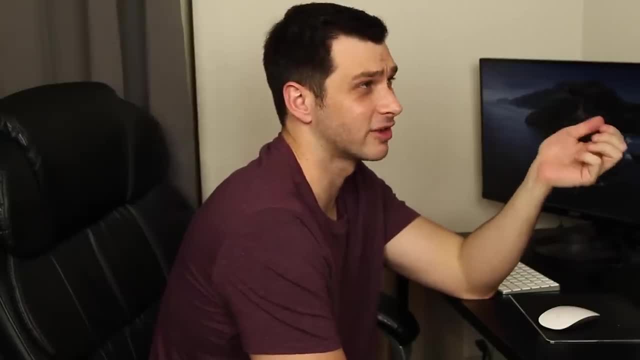 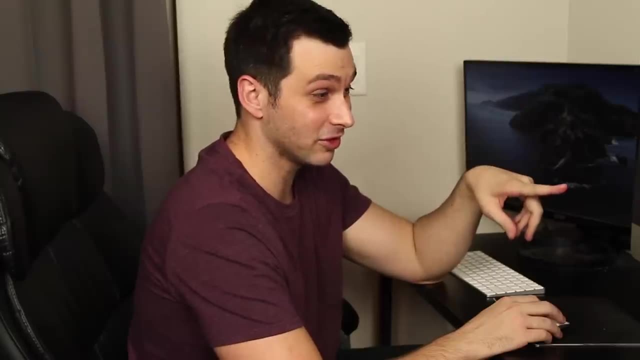 I'd say finishing two programming assignments in one night is the closest I've been to a threesome. I asked if you were done on the computer. In fact I programmed hello world before I could say hello world. I mean like hey, you're catching up. 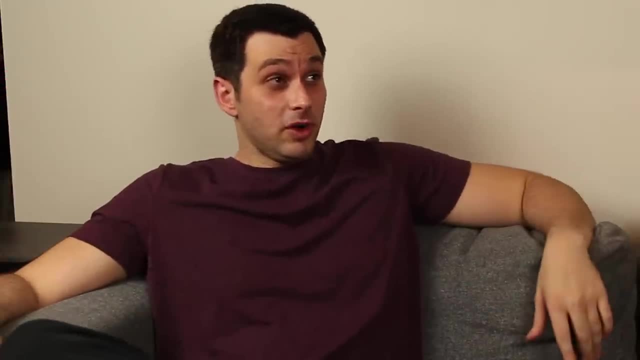 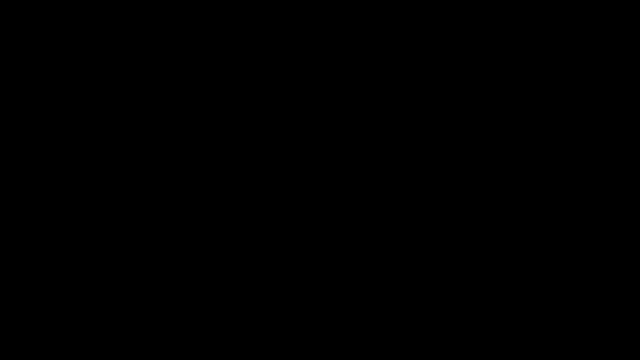 I'm just saying, if you use a lookup table, you're a bitch. Oh my God. Yeah, I heard you Now for the last time. what do you want on your pizza? All right, you take that one. I think we're good.